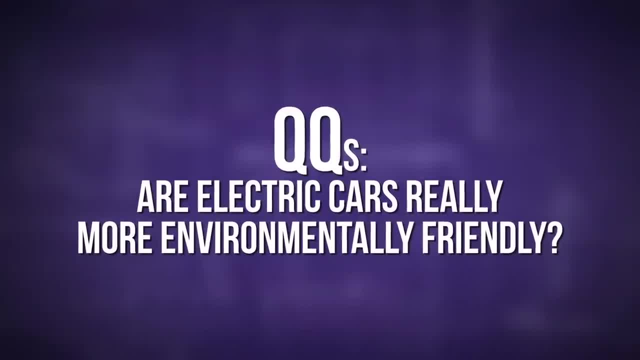 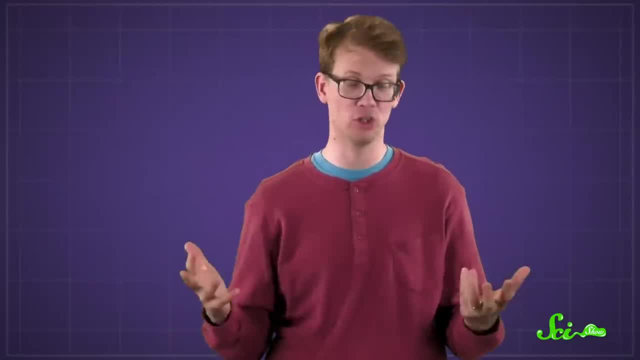 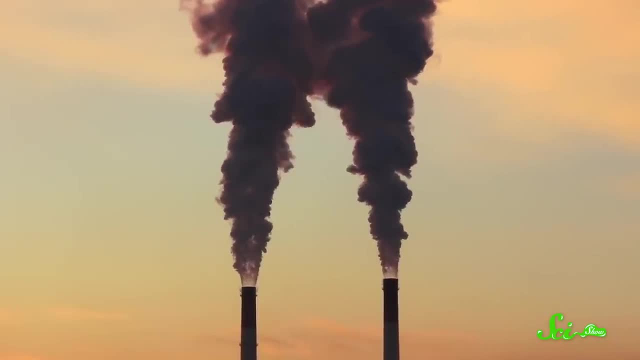 Telling people that buying an electric car is a great way to fight climate change is a pretty reliable way to start an argument. in some circles People will say that you still burn fossil fuels with electric cars. it just happens at the power plant instead of the engine. And while that is at least partly true, over their lifespans electric cars don't consume anywhere near the fossil fuels that gas-powered cars do, especially in the United States. With electricity getting cleaner all the time, they're even better than you might expect. 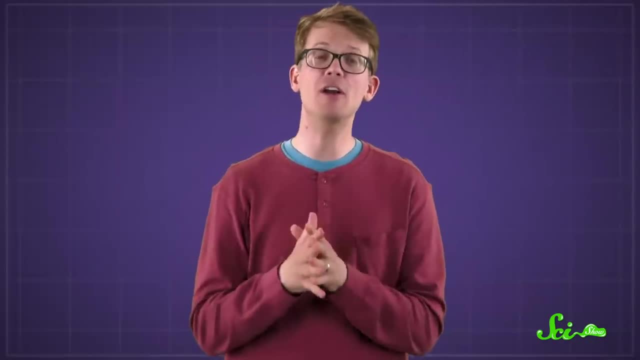 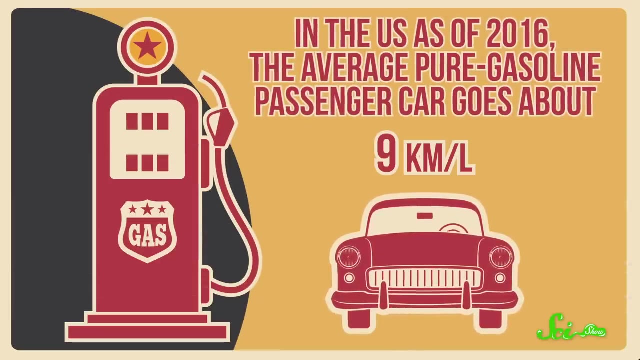 There are a few variables to keep in mind, though, starting with the cars themselves. In the US, as of 2016,, the average pure gasoline passenger car goes about 9 kilometers for each liter of gas it burns, or about 22 miles per gallon. 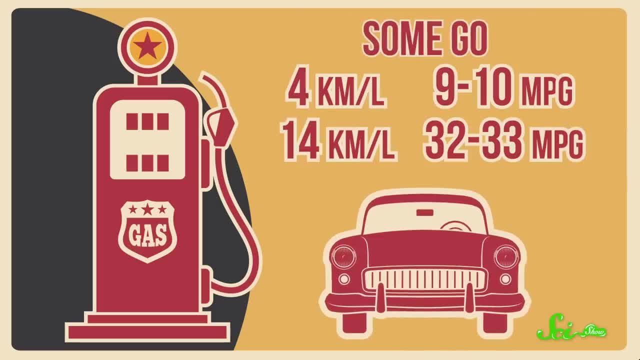 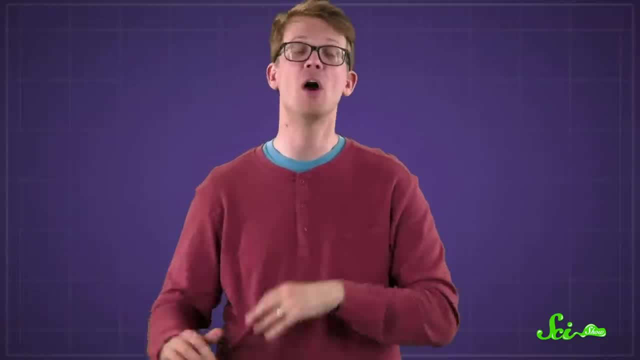 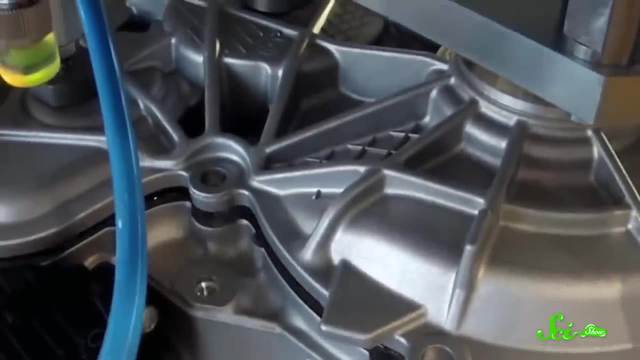 But that's just an average. Some go 4 kilometers or so, others go 14.. But the fuel efficiency hits higher highs and lower lows when we're talking about hybrids, cars or trucks on the interstate. Plus, the act of manufacturing a car leads to greenhouse gas emissions, whether it's electric or not. So does refining gasoline. The major complicating factor here is electricity, and where you live determines how clean your electricity really is. Most electricity in the US uses a combination of natural gas, coal and nuclear fission, with a bit of water, wind, solar oil and a few others thrown in. 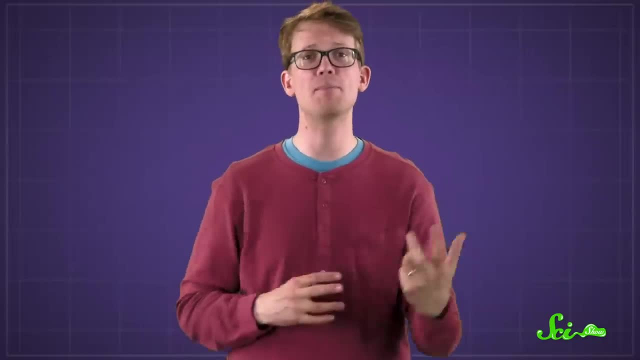 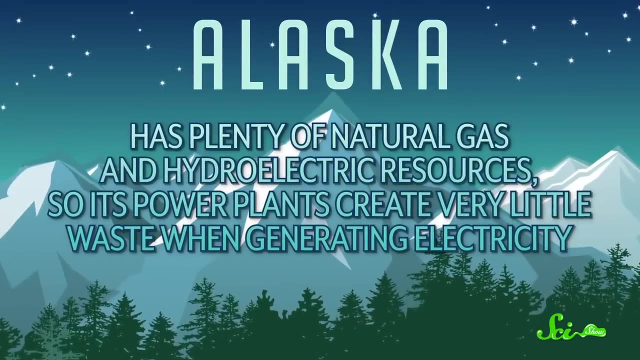 But those numbers change from state to state And depend on things like local natural gas sources or how windy it is. today, For example, Alaska has plenty of natural gas and hydroelectric resources, so its power plants create very little waste when generating electricity. 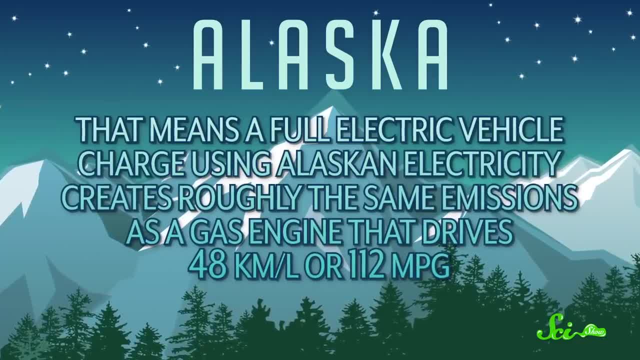 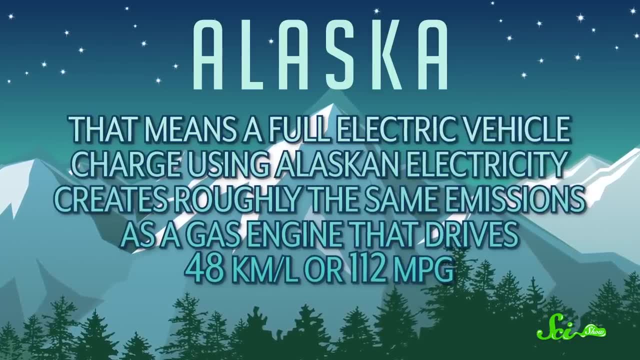 That means a full electric vehicle charge. using Alaskan electricity creates roughly the same emissions as a gas engine that drives 48 kilometers per liter or 112 miles per gallon. That's roughly five times the national average And two or three times bigger than that. 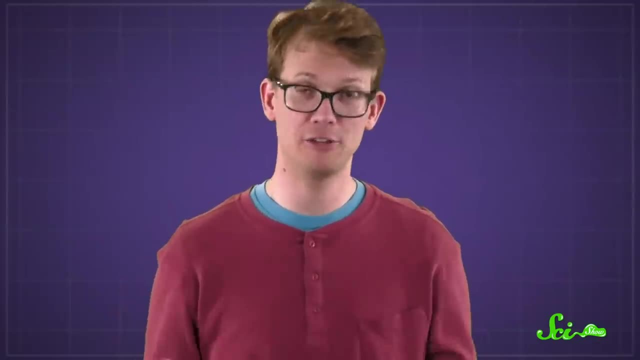 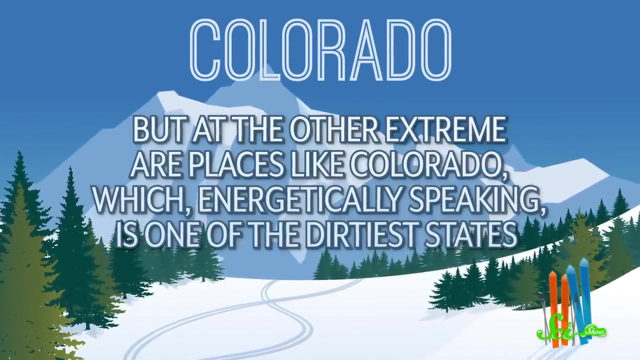 Two or three times better than even some of the best hybrids. It's pretty efficient. But at the other extreme are places like Colorado, which, energetically speaking, is one of the dirtiest states. Sorry, Colorado. About half of Colorado's electricity is from coal, which produces more emissions than just about any other source. 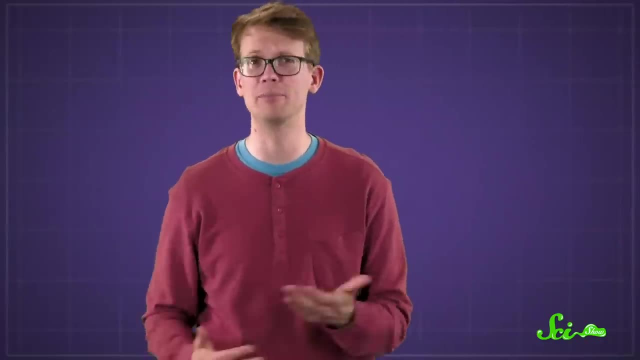 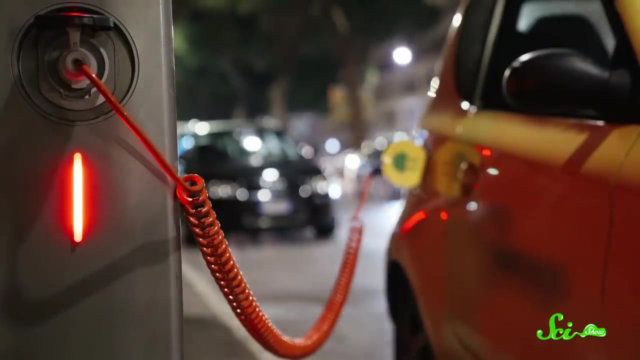 But even there, electric cars still outperform gas cars. A full charge off of Colorado electricity equates to about 20 kilometers per liter, 46 miles per gallon. That's about double the national average based on 2016 figures. That's pretty good. Better still, most of the country is closer to Alaska's numbers than Colorado's. It comes down to this: Power plants are just better at making power than car engines are. One reason is that they're simply bigger. Bigger things don't waste as much energy staying hot, and that makes them more efficient.